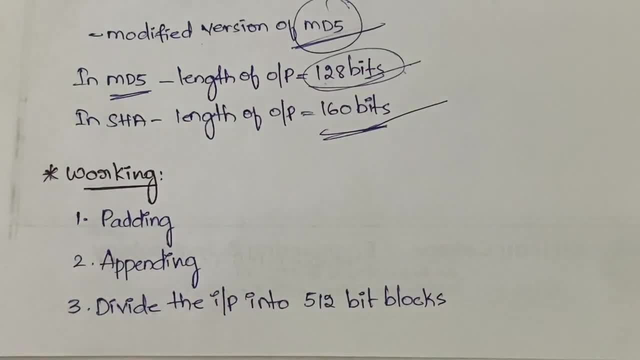 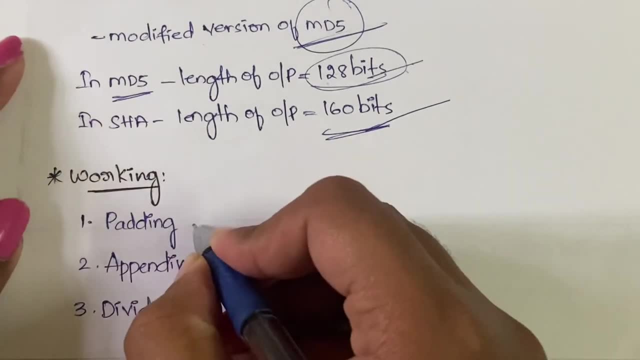 moving on to the working, In working we have different steps, as we have in MD5. So the similar steps we have first is padding right. Padding what you will do is it is also same as MD5. again, That is why I said you to watch MD5 videos. It should be 64-bit, 120-bit. 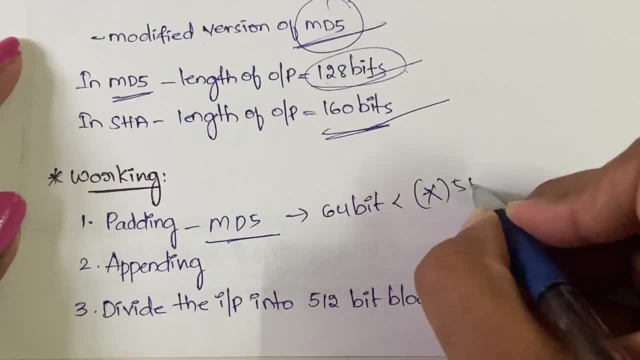 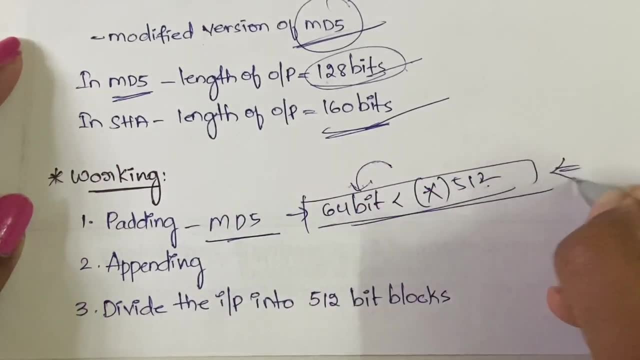 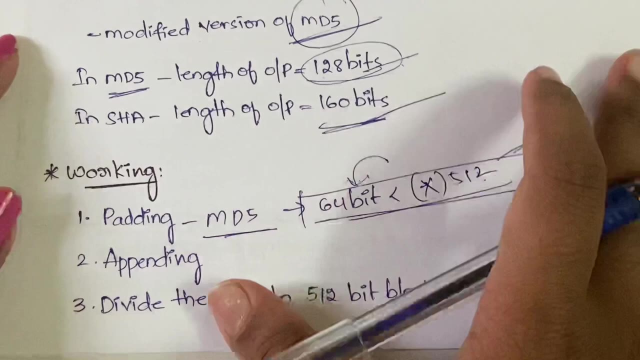 less than exact multiple of 512.. Got it. It has to be 64-bit less than exact multiple of 512.. What it means: The total length. The total length should be so, depending on this. according to this, you need to add the padding bits at the end. Got it? So the first and 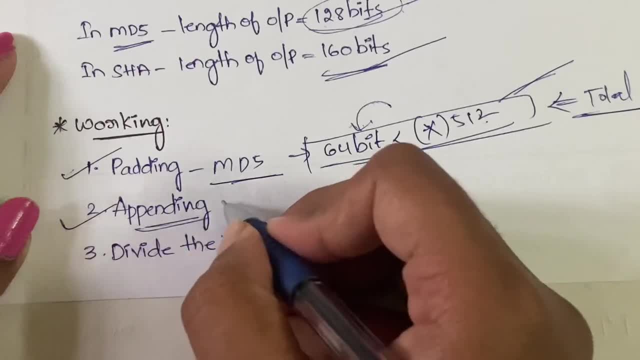 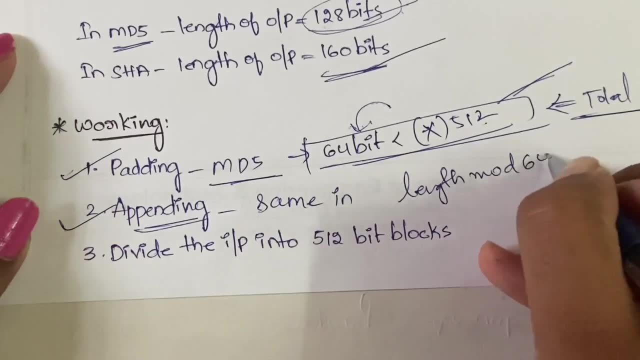 second step is appending In. appending also the same, the same how you did in MD5, the same you have to do Length mod 64, we did right The same step. you have to follow here as well. Now, in the third, 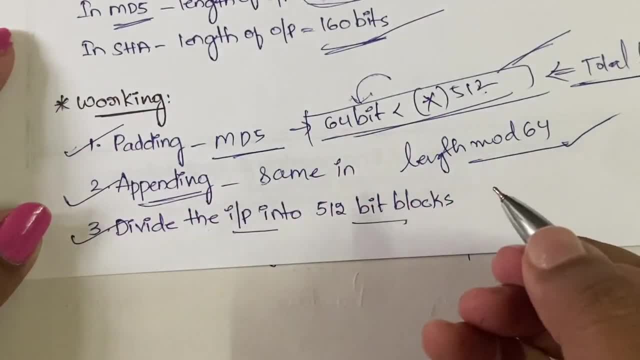 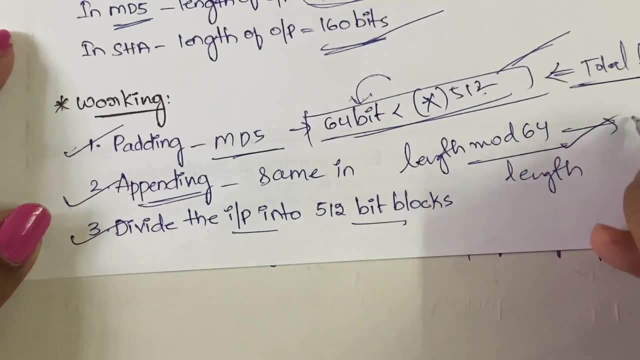 step. what you are doing? you are dividing the input into 512-bit blocks. The same again. we did the same thing in MD5 as well. In MD5, the total length after appending it will obviously become the multiple of 512, right After appending. Now you need to divide this. 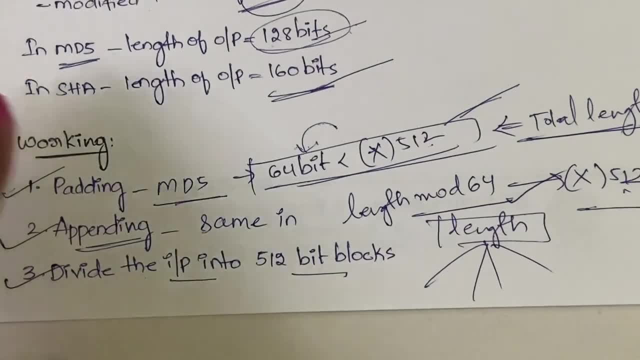 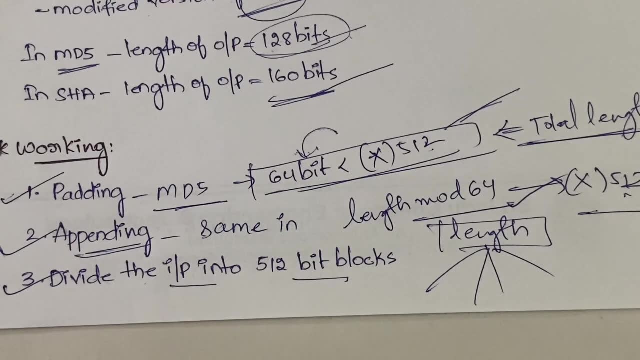 length into number of 512-bit blocks. Okay, So up to here, everything is same as MD5. These three steps are almost- not almost Completely- similar to MD5.. The only thing you are going to observe the changes in the. 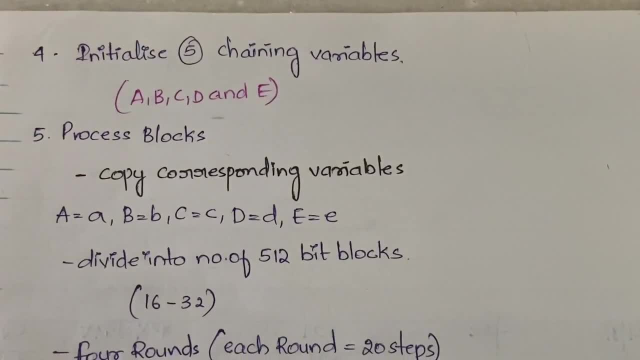 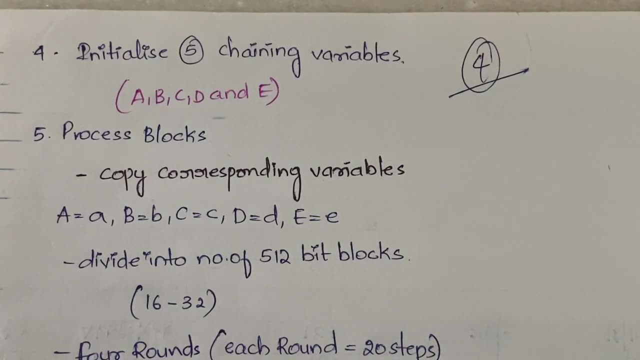 case of fourth step. In the fourth, in the case of fourth step, you, what you will do is in MD5, what we did, we initialized four chaining variables, right, But here we are going to initialize five chaining variables. Got it Five: A, B, C, D and E. We are going. 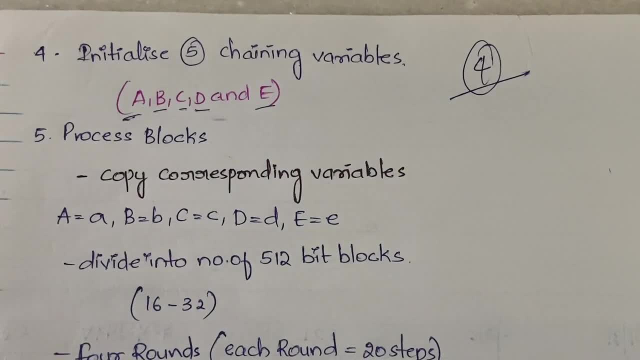 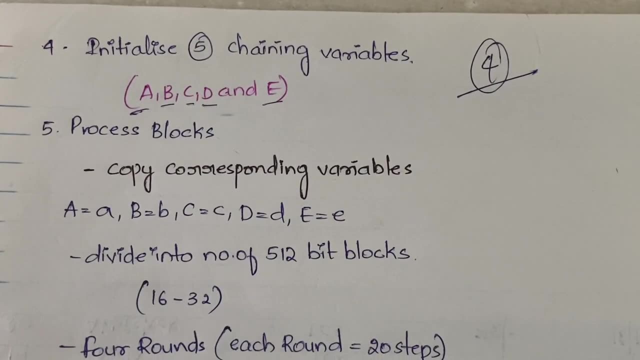 to initialize total of five chaining variables in this. Next, in the second step, in the- I mean the last step where we do the processing- again copy the corresponding variables: a is equal to a, b is equal to B, like that you will. 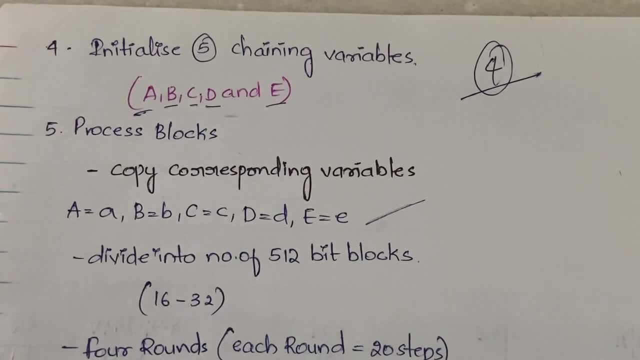 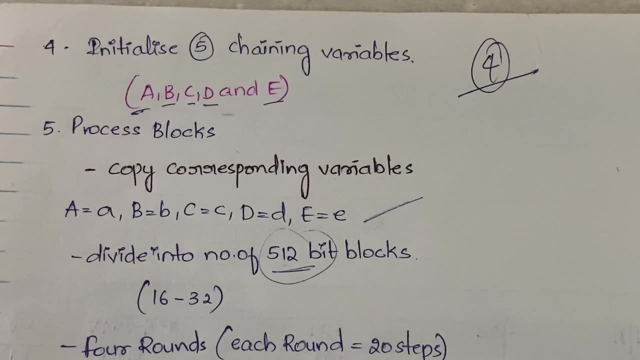 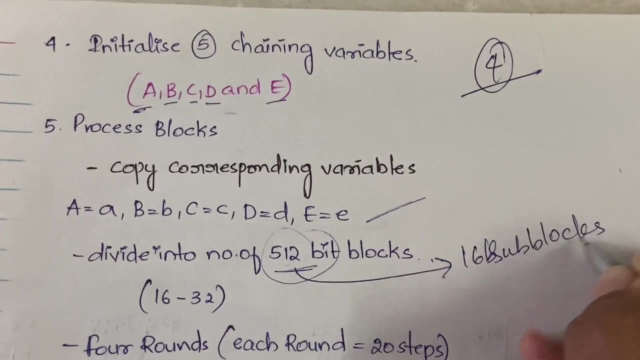 be copying the corresponding. So once you are done with copying, then what we will do? We will be dividing each and every 512-bit sub-block into 16 32-bit blocks. That is, you will be dividing 512 x 16 sub-blocks and the size of this, each and every sub-block. 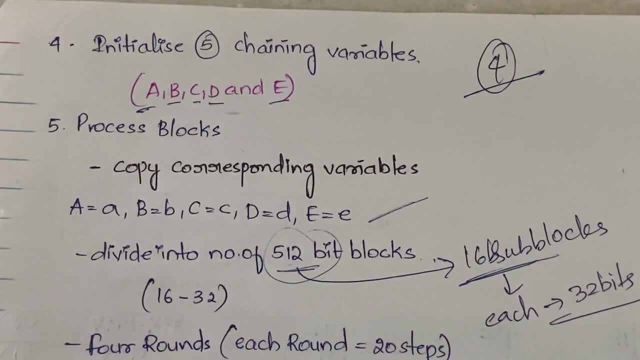 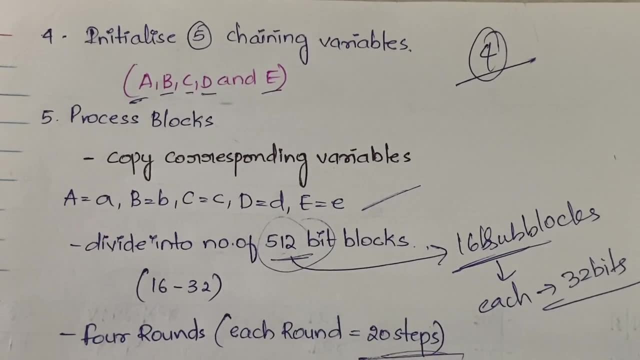 will be equal to 32 bits. Got it? So this is how you do. Next, again, you will be performing four rounds. in each and every round, you have total of 20 steps. you need to perform total of 20 steps in each and every round like that. how many rounds you have to do? you need. 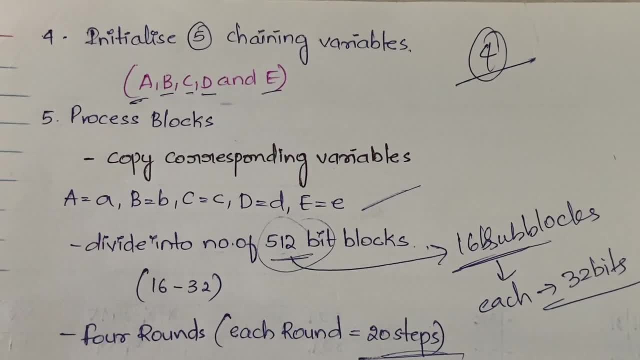 to do four rounds got it. so this is all about sh algorithm. of course i know the video is very short because it is completely depending on md5. for the step one, two, three, you can write whatever theory that you have written for md5. you can write the same thing in case of fourth step, the only. 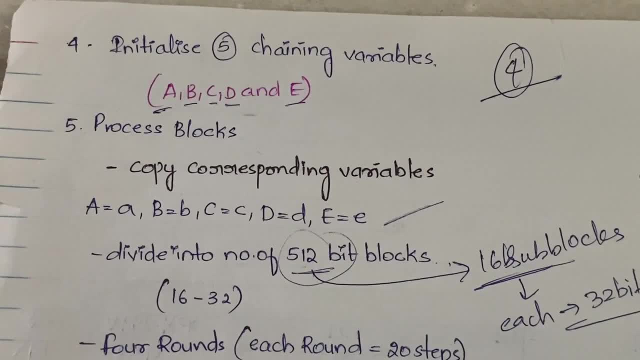 thing that is going to change is: there you initialize four chaining variables. here, you initialize five chaining variables, and even the fifth step also, it is going to remain the same. got it? so this is about sh, a secure hash algorithm. what is the purpose of this algorithm for? 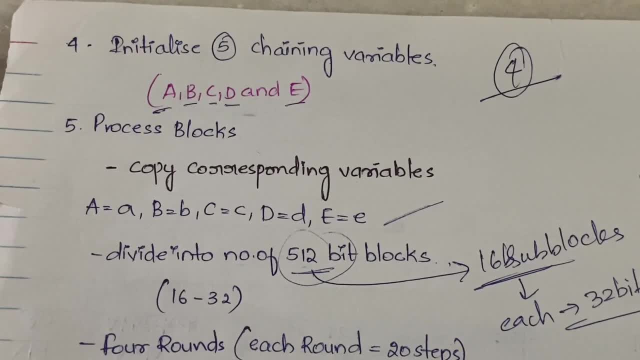 authentication. and in authentication, what we have? we have hash based functions, we have message authentication codes- right. we have encryption right. so in hash based code we have md5 and secure hash algorithm right. and again in the category of message authentication, we have hmac, cmac and all. 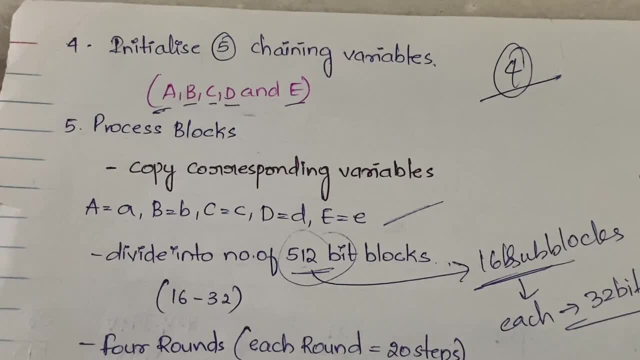 i will explain about them in the next coming videos. got it? so this is all about sha in sha. you will have total of five steps. in the first step you have to do padding, padding such that the original length, the total entire length, will become 64 bit less than the multiple of 512. 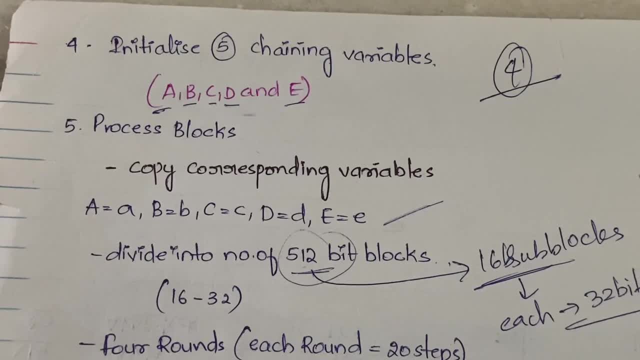 in the second step, you will be doing the appending. in the third step, you will be dividing it into number of 512 blocks. in the fourth step, you will be having taking some chaining variables. in the fifth step, you will be processing those chaining variables. you will be 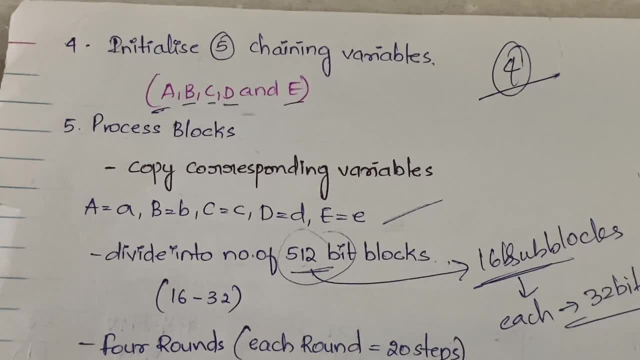 dividing again 512 into 16 blocks, each of size 32 bits, got it. so this is all about the secure hash algorithm, and if you're still having any doubts apart from what i've explained in this video, you can let me know in the comment section so that i will try to clear all your doubts. for 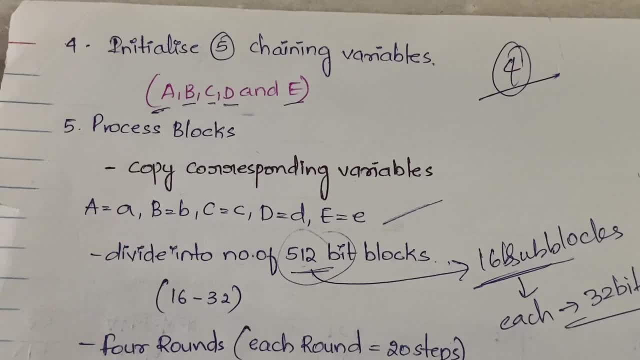 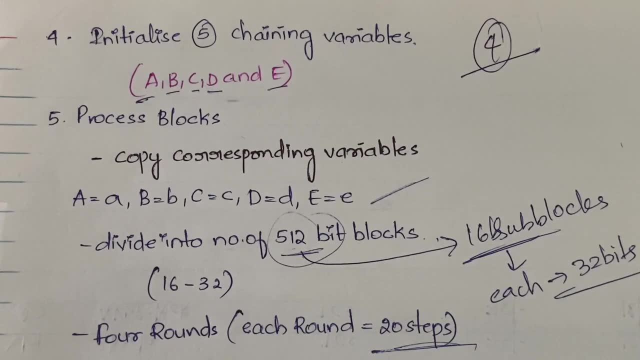 sure, and if you're having your exam schedule nearby, just let me know the date of your exam in the comment section so that i can make videos by your exam date, got it? so let's stop this video at this point and let's meet up in a second in the other videos. you.